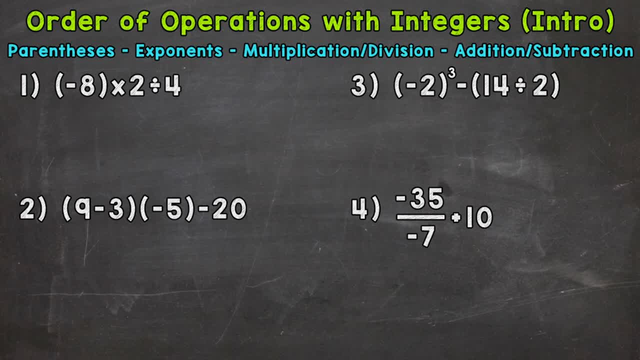 have any sets of parentheses where we have to solve something within those parentheses? No, We do have parentheses, but we just have a negative 8 in there, Nothing that needs to be solved. We sometimes put parentheses around negative integers to help us solve the problem, But we don't have to solve the problem. We don't have to solve the. 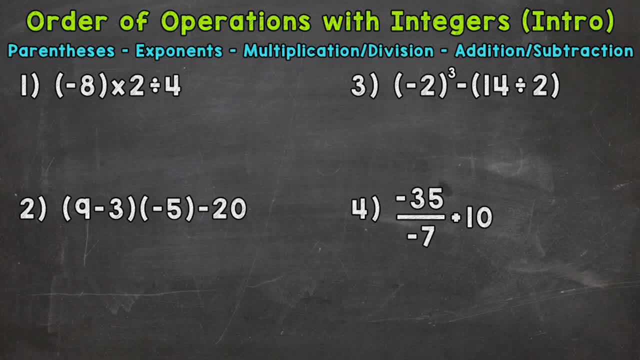 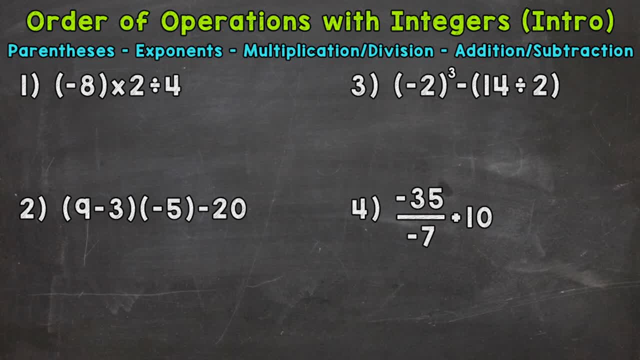 negative 8 stick out so we don't forget it's a negative 8 and lose sight of that as we go through our process. So we now go to exponents- Any exponents, No, Any multiplication or division: Yes. So that's where we start. Negative 8 times 2.. So we have a negative times a positive A. 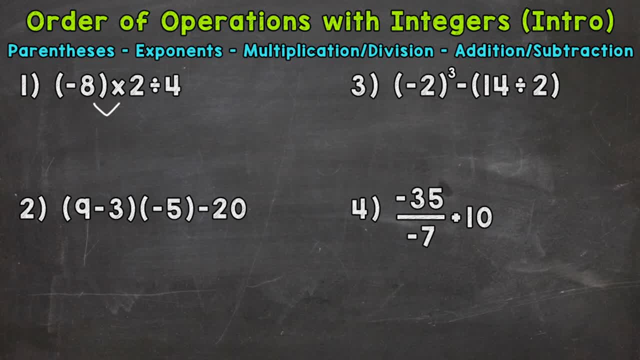 negative times. a positive equals a negative, So this is going to be negative 16.. Bring down everything we did not use, So the division and the 4.. So we end with negative 16 divided by 4.. A negative divided by a positive equals a negative. So this equals negative 4 and that's. 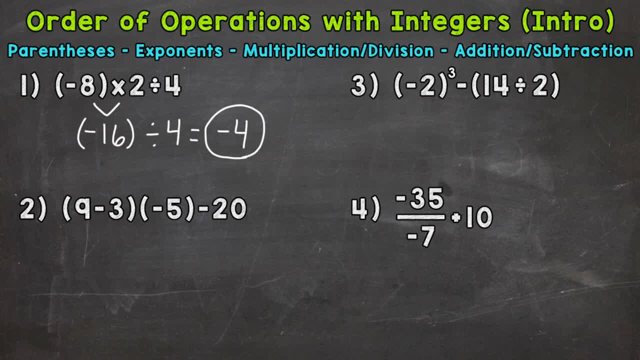 going to be our answer. Let's go on to number two, where we have parentheses 9 minus 3, end parentheses. times negative: 5 minus 20.. So let's go through our process: Any parentheses where we have something to solve within the parentheses: Yes, 9 minus 3, which equals 6.. Bring down everything. 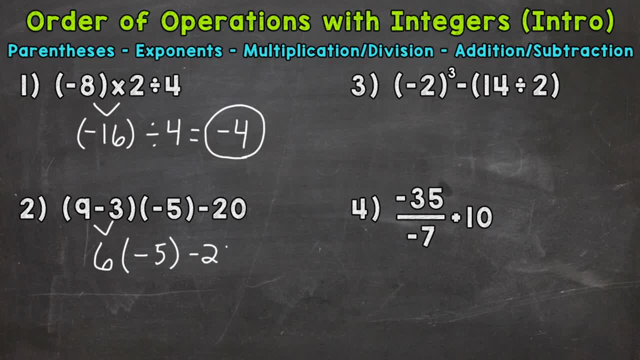 we did not use and go from there. So any parentheses where we have something to solve. No, Any exponents, No Any multiplication or division. Yes, So that 6 next to the parentheses, that means multiplication. So we have 6 times negative, 5. So a positive times a negative equals a negative. So this is going to be. 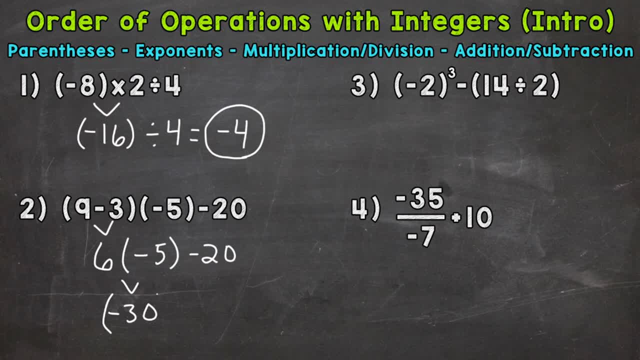 negative 30. Then we bring down our subtraction and the 20. So we have a negative equals a negative. So this is going to be negative 30. So we bring down our subtraction: negative 30 minus 20.. So what we can do here, we can add the opposite. That helps us subtract. 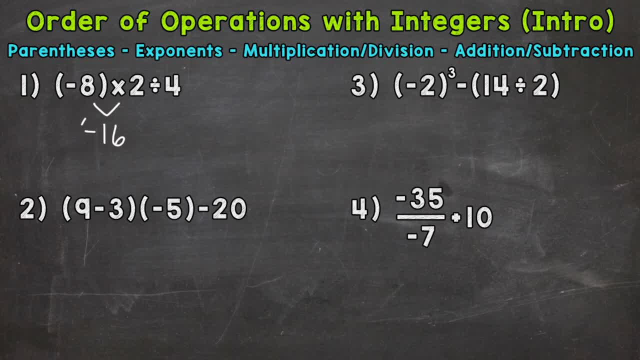 So this is going to be negative 16.. Bring down everything we did not use, So the division and the 4.. So we end with negative 16 divided by 4.. A negative divided by a positive equals a negative. So this equals negative 4 and that's going to be our answer. 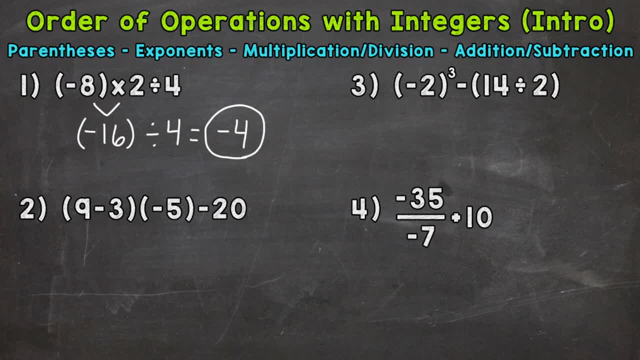 Let's go on to number 2, where we have parentheses 9 minus 3, end parentheses: times negative: 5 minus 20.. So let's go through our process. Any parentheses where we have something to solve within the parentheses: Yes: 9 minus 3, which equals 6.. 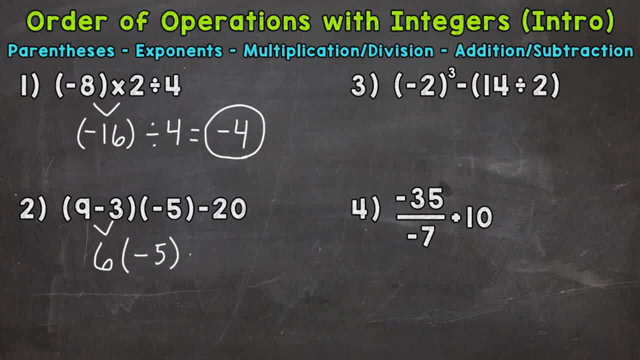 Bring down everything we did not use And go from there. So any parentheses where we have something to solve, No, Any exponents, No Any multiplication or division. Yes, So that 6 next to the parentheses, that means multiplication. 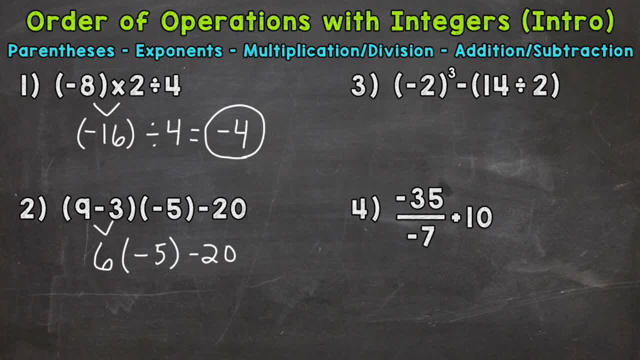 So we have 6 times negative 5. So a positive times a negative equals a negative. So this is going to be negative 30. Then we bring down our subtraction and the 20. So we have a negative 30 minus 20.. 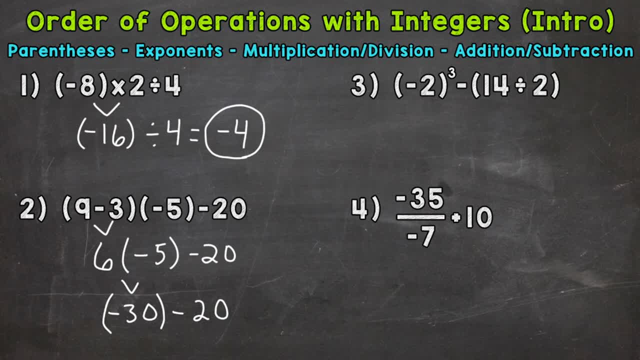 So what we can do here? we can add the opposite. That helps us subtract integers. So let's add a negative 20. So that's going to give us negative 30 plus negative 20 is negative 50. Again, we added the opposite. 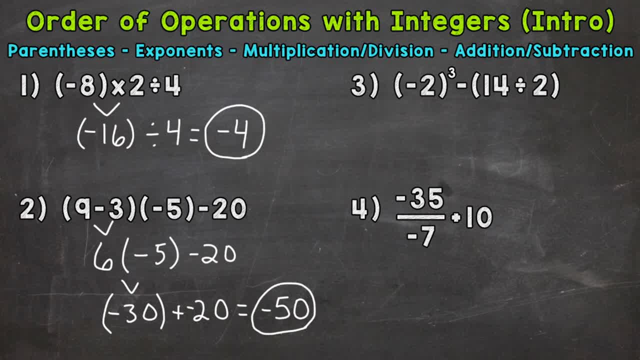 If you like to think of it as negative 30 minus 20, you're subtracting 20.. You're going 20 to the left down the number line. That works. That works too. You're still going to end up with negative 50.. 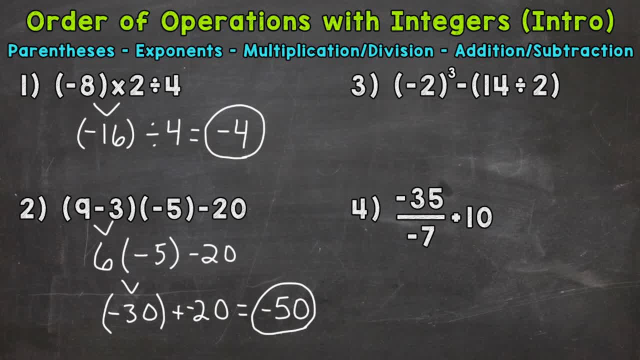 But again, you can also add the opposite. when it comes to subtracting integers, Let's move on to number 3, where we have negative 2 cubed, or negative 2 to the power of 3 minus parentheses, 14 divided by 2 and parentheses. 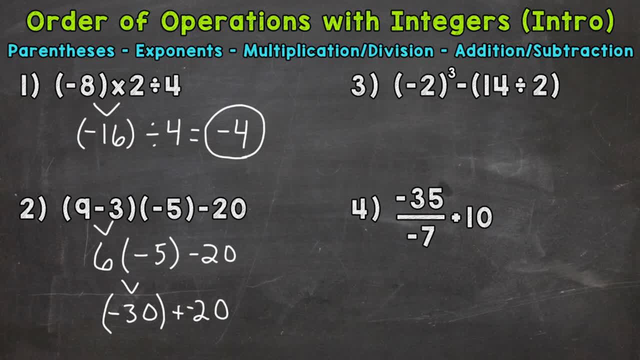 integers. So let's add a negative 20.. So that's going to give us negative 30 plus negative 20 is negative 50.. Again, we added the opposite, If you like to think of it as negative 30 minus 20,. 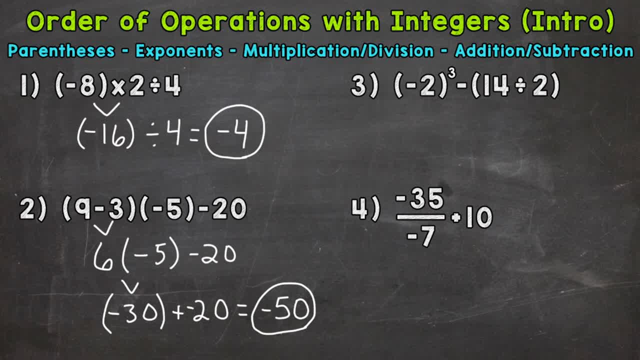 you're subtracting 20, you're going 20 to the left down the number line. That works too. You're still going to end up with negative 50. But again, you can also add the opposite. when it comes to subtracting integers, Let's move on to number three, where we have negative, two cubed or negative. 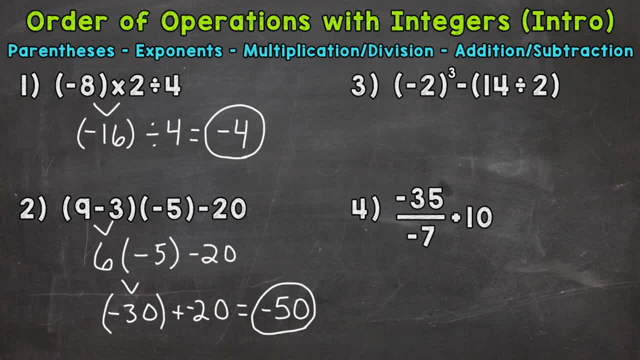 two to the power of three minus parentheses. 14 divided by two and parentheses. Let's go through our process, So any sets of parentheses. let's go through our process, So any sets of parentheses where we have something that needs salt. Yes, the 14 divided by two. we will start there, So 14. 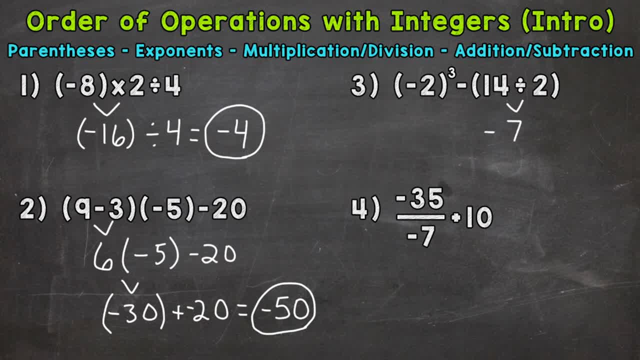 divided by two is seven. Bring down everything we did not use. So any parentheses where we have something to solve. No, Any exponents. Yes, we have negative two cubed, So that means negative two times negative, two times negative two. And then we add the opposite. So we add the opposite. 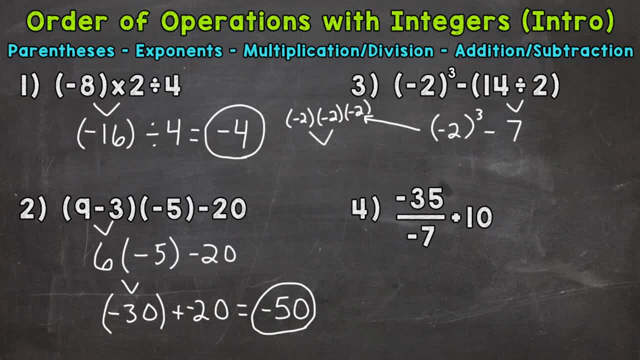 So any parentheses where we have something that needs salt: Yes, the 14 divided by two, we will start negative 2. so negative 2 times negative 2. a negative times a negative equals a positive 4. bring down the other negative 2 so we end with a positive 4 times a negative 2, so that's going. 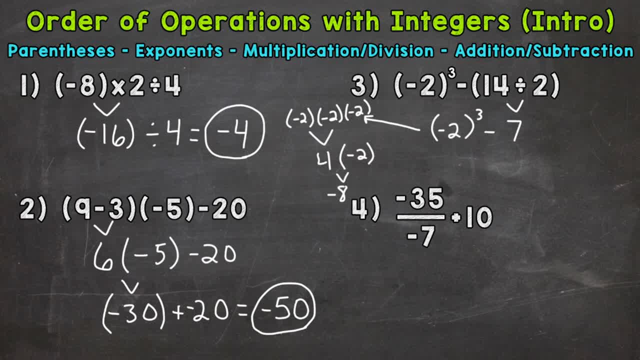 to give us a negative 8, because a positive times a negative equals a negative, so this is negative 8 here. bring down the subtraction and the 7. so, just like number two, we have a negative and we are subtracting a positive, so we can add the opposite. let's add the opposite here. 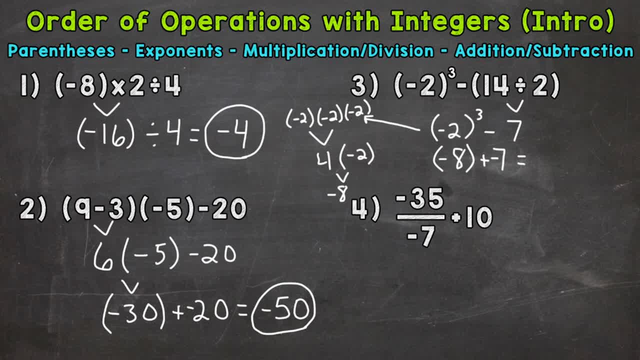 and we end up with negative 8 plus negative 7, which equals negative 15. and lastly, number four: we have negative 35 divided by the number of times a negative 7 times a positive 6, and now we have a negative by negative 7 plus 10.. So, any parentheses, No, Any exponents, No Any multiplication or division.